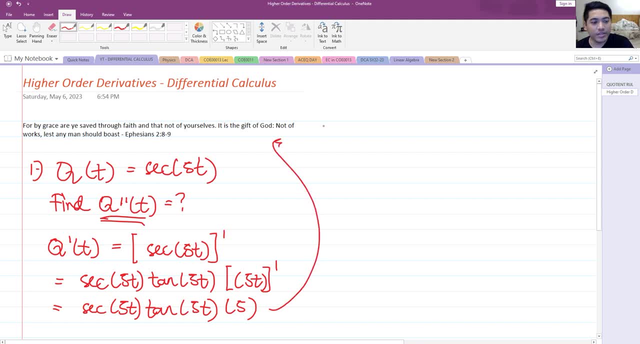 to t would be 5.. So now we are left with the first derivative as 5 secant of 5t, and then we have tangent of 5t. All right, so that's the first derivative. So how about the second derivative? 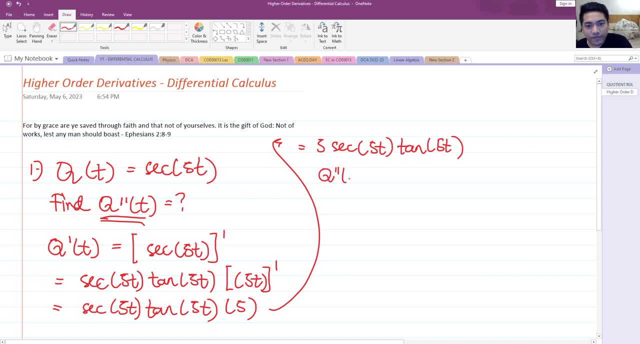 So if we're going to get the second derivative of secant of 5t, we're going to get the second derivative of secant of 5t. So the derivative of this. okay, let me just first factor out 5.. Okay, so just just factoring it out. 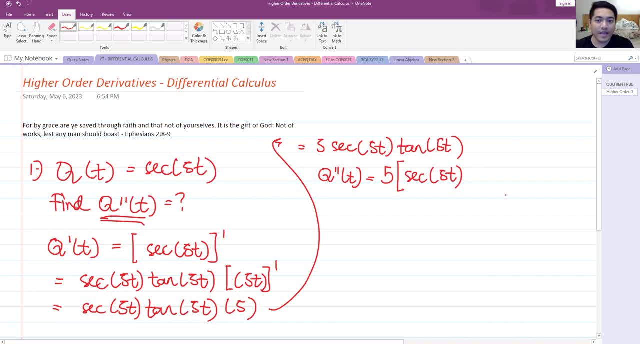 outside the bracket because secant 5t, tangent 5t. what we are going to do with that is to use product rule, So I'll just have the 5 outside of the bracket. Okay, so I'm going to do that. get the derivative of that. That is product rule. 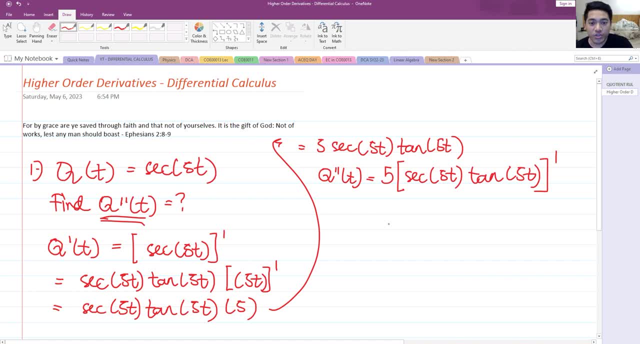 So the product rule suggests that you have UDV plus VDU or just like from my previous videos, we can copy the first one, secant 5t, and then we're going to differentiate tangent of 5t- Okay, differentiate that, Okay. and then we have plus- Okay, copy tangent of 5t. Copy this. 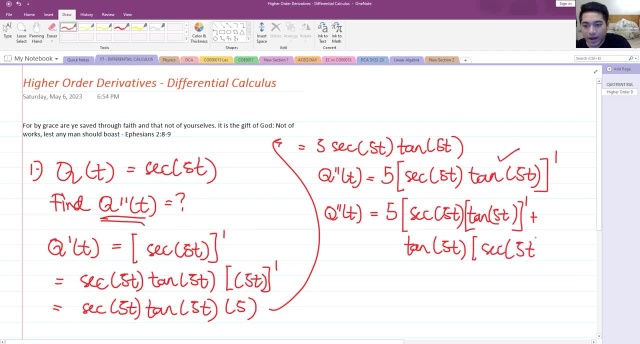 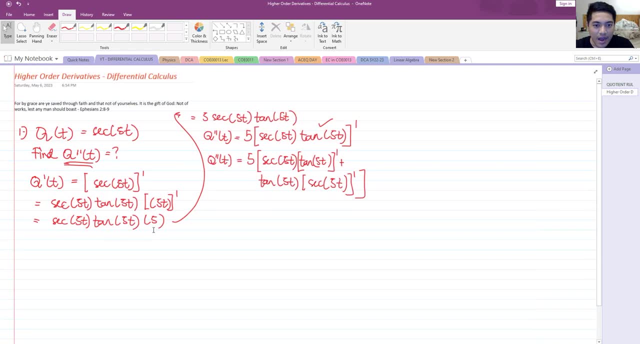 and we're going to differentiate that, Okay. and then we have plus: Okay, copy tangent of 5t, Copy this, and we're going to differentiate that secant of 5t, okay. so now we have applied the product rule, so let me just have some space here. 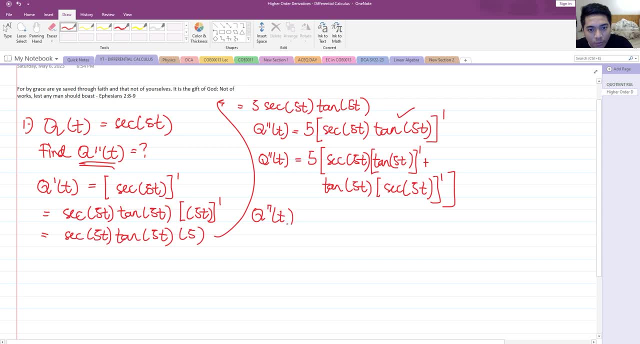 okay. so if we do that, we have 5 multiplied on the derivative of the whole secant 5t and tangent 5t. don't forget that. so we have secant of 5t multiplied by the derivative of tangent 5t, the derivative of tangent 5t, secant squared 5t. and of course, don't forget to differentiate again. 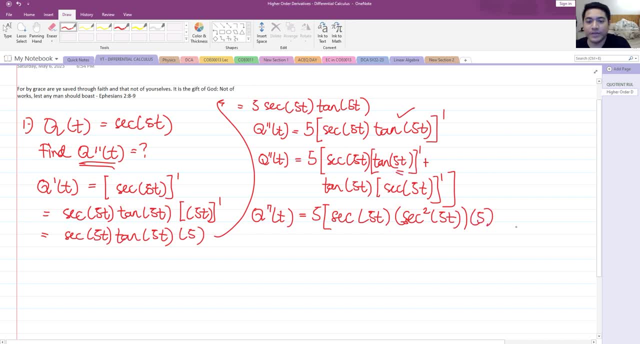 the 5t, so we will be having 5 here. okay, so that's the derivative of tangent of 5t. we have secant squared of 5t multiplied by 5. okay, so we have used chain rule for that. so then, plus, we have: 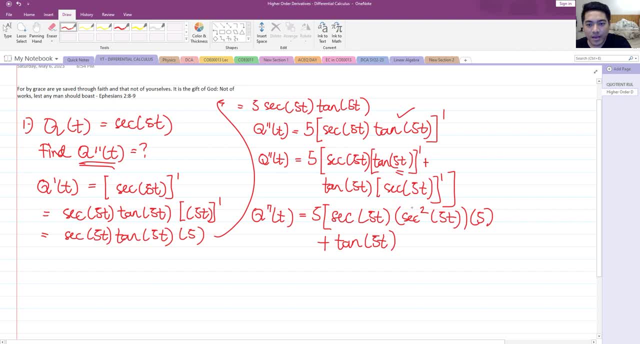 tangent of 5t. okay, derivative of secant 5t, secant of 5t is the same. so we have seen that a while ago here, that the derivative of that is 5, secant 5t, tangent 5t. so that becomes 5, secant of 5t and then tangent of 5t. okay, so let me just 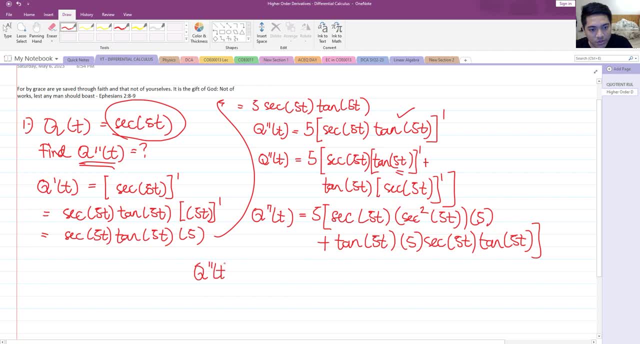 rewrite the whole equation, the whole solution. so we have: okay, we are going to distribute 5 on this term and also on this term. okay, so we have factored out 5 a while ago so that our differentiation will be easier. okay, so if I'm going to do that, that's 5 times 5. we have 25 secant of 5t, and then we have 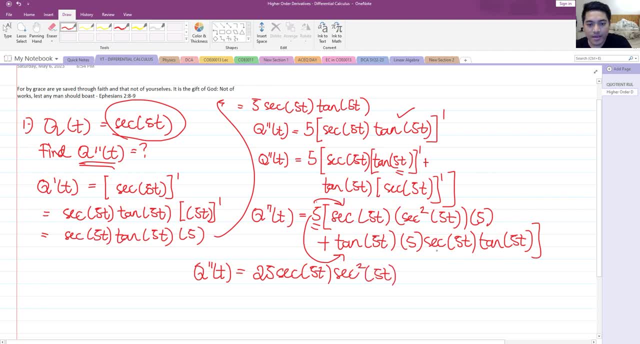 secant squared of 5t plus we have 5 times 5 the same. okay, we have secant of 5t. this one tangent times tangent, that becomes tangent squared of 5t. so I just forget this can be also multiplied: secant 5t and secant squared of. 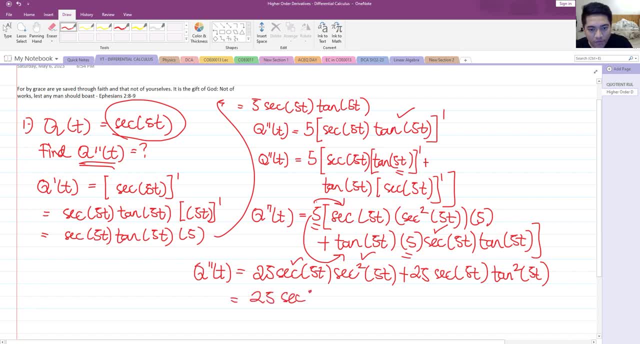 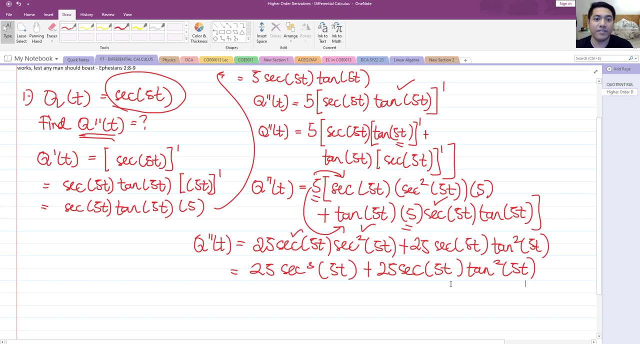 t. so we have 25 secant of cube of 5t and then we have plus 25 secant of 5t and then tangent squared of 5t. so that is our answer for getting the second derivative of secant of 5t. however, we can still. 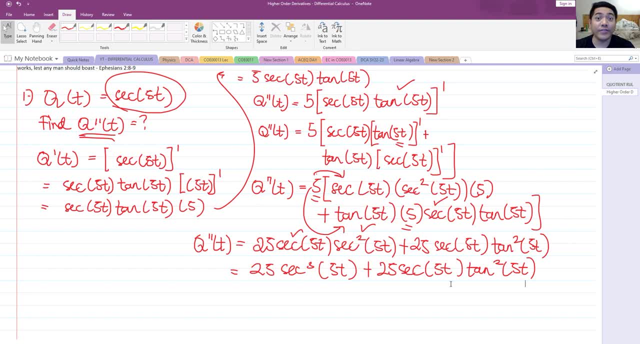 simplify the final answer by factoring out some common factors. so we have- you can see, we have 25 here common factor. we have secant here common factor, so we have 25 secant of 5t. I'm going to factor it out. so what's left for this term will be secant squared of 5t, and then we have plus tangent squared. 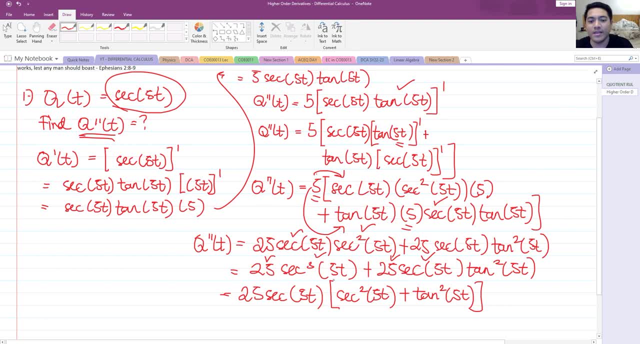 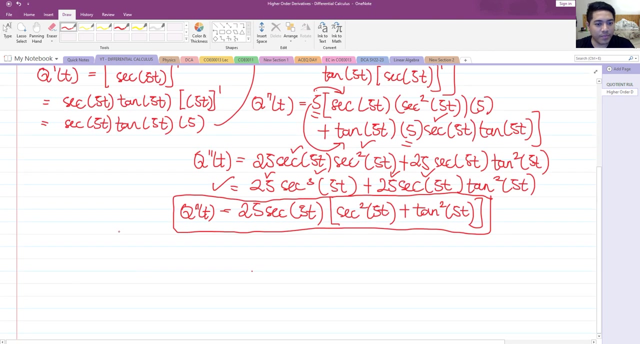 5t, so that if you multiply 25 secant 5t, we can arrive at this answer still. so this is just the simplified okay answer for our second derivative of q of double prime of t. okay, so that's our answer. all right, let's go now to the second problem. so we have for the second problem. 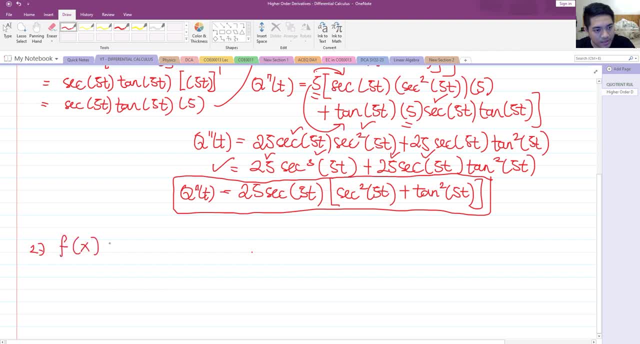 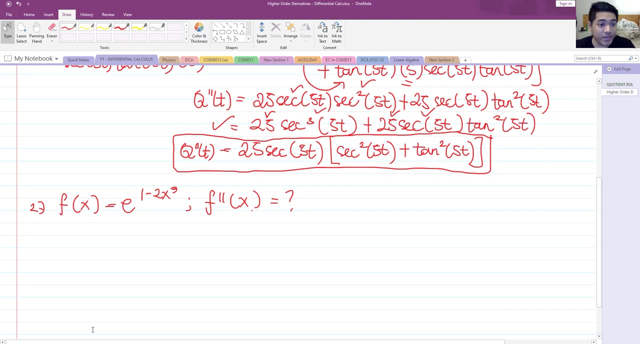 we have f of x equals e raised to 1 minus 2x cube and we're going to get the second derivative of that f of x. so, if we may recall that the derivative of exponential function is simply the derivative of the exponent multiplied by the original function, okay, so let's write first to get: 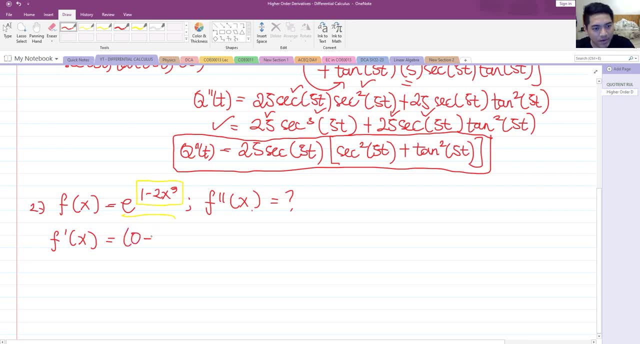 f, prime of x. so that would be zero. so that would be zero minus 6x squared multiplied by the original function f of x. so zero minus 6x squared because we differentiated the exponent of which that becomes zero minus 6x squared because of the. 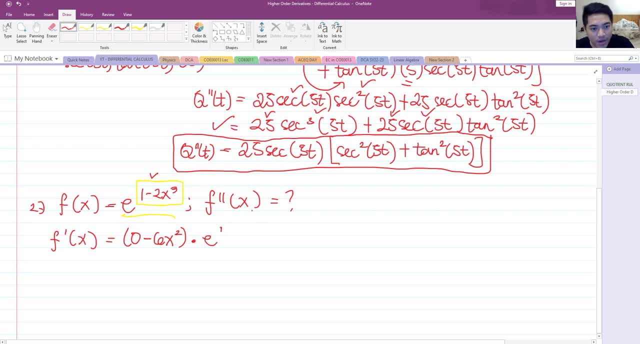 power rule. so we have e raised to 1 minus 2x cube. so, simplifying, we have negative 6x squared multiplied by e raised to 1 minus 2x cube. so that's the first derivative. so that's the first derivative. so in the second derivative we will shall be repeating the process. f- double prime of x. 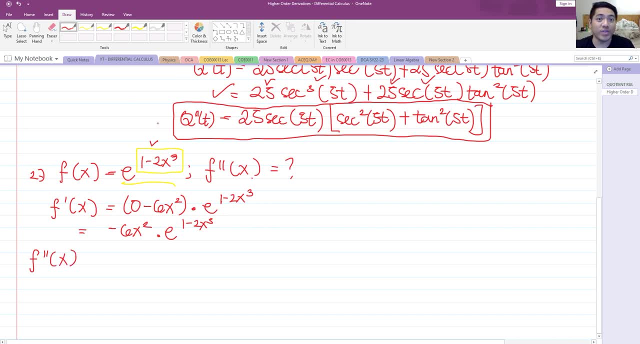 so what technique do we need to use in order for us to get that? so we are going to use product rule, as this is an algebraic function multiplied by an exponential function. so we're going to get okay. first copy negative 6x squared and then multiply it by the derivative of e raised to 1. 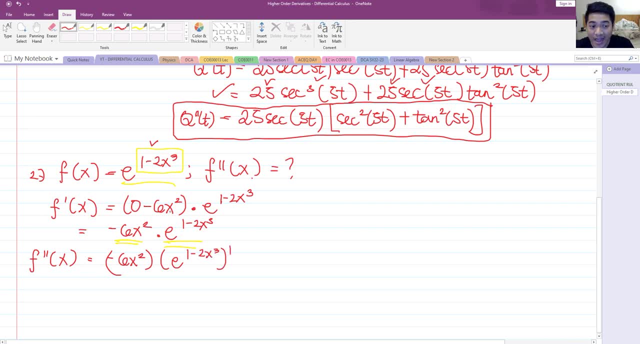 minus 2x cube, of which that's the original function. so we're going to use product rule, as this is an algebraic function. so we're going to use product rule, as this is an algebraic function that we had a while ago. then plus copy the second function, which is the exponential function. so we 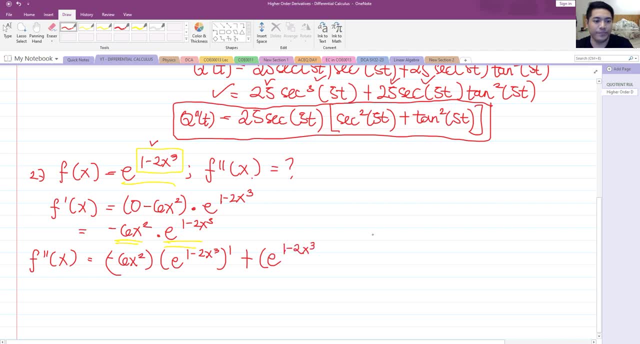 have e raised to 1 minus 2x cube, multiplied by the derivative of the first, which is negative 6x squared. okay, so, as we all know, we have already differentiated this as this is the original function. so we have negative 6x squared multiplied by the derivative of the first, which is negative 6x squared. 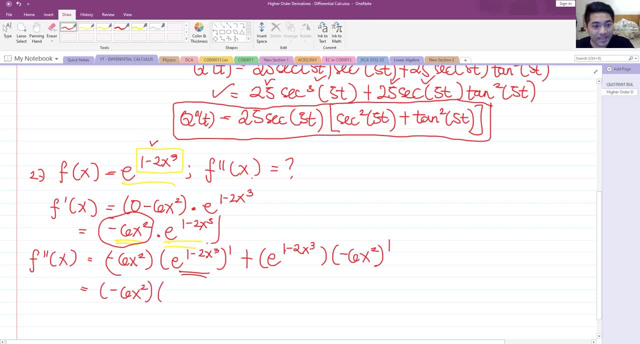 by the derivative of e raised to 1 minus 2x cube. is this result that we have solved a while ago, so that becomes negative. 6x squared e raised to 1 minus 2x cube. plus e raised to 1 minus 2x cube. 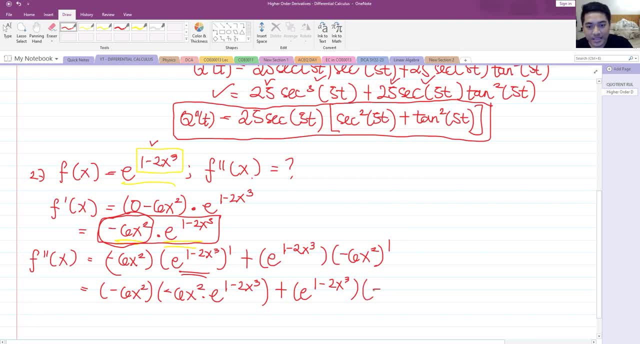 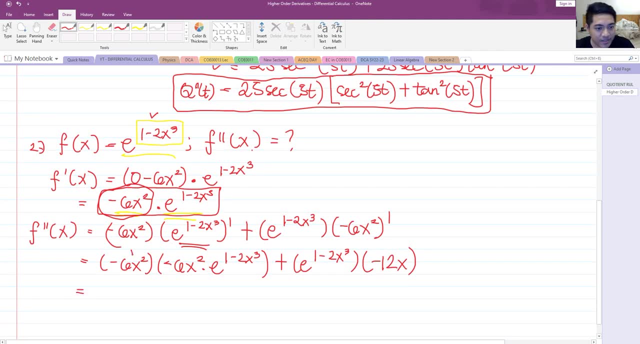 multiplied by the derivative of negative x 6x squared, that's negative 12x okay. so simplifying negative 6x squared times negative 6x squared, that becomes positive. so we have 36x raised to 4, e raised to 1 minus 2x cube, okay. and then negative 12x times e raised to 1 minus 2x cube. so 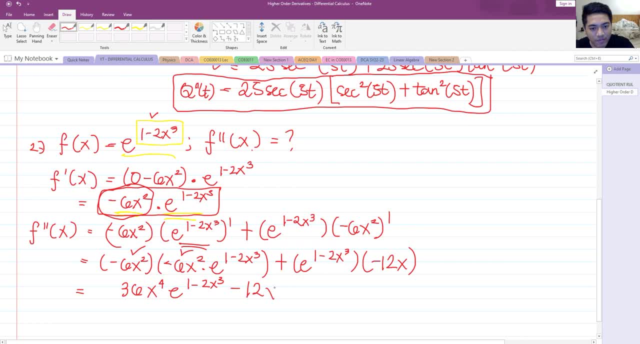 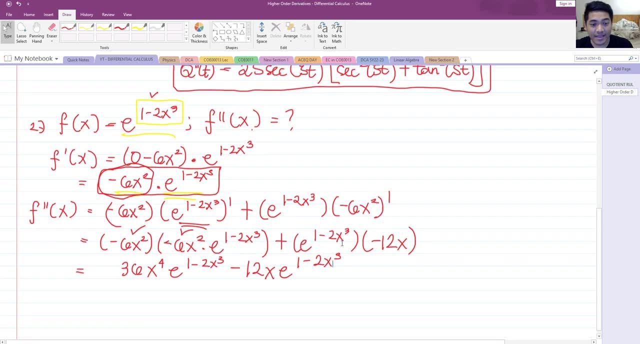 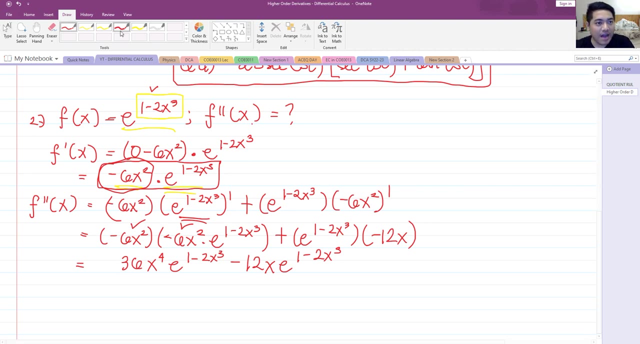 negative and then positive, that becomes negative. 12x e raised to 1 minus 2x. okay, so we can still simplify by factoring out common factors from the two terms that we have. so we have a common of 12 and 36 is divisible by 12. 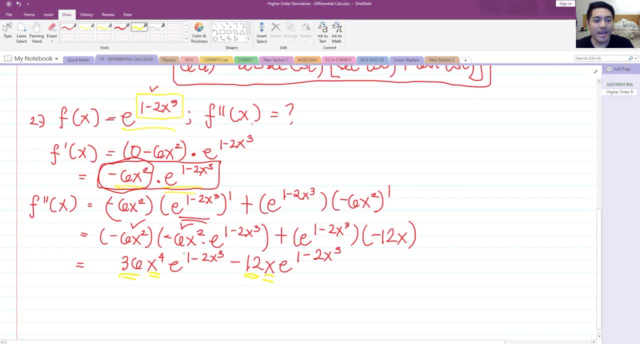 and we have a common factor of x here and e raised to 1 minus 2x cube. so we can factor that out. so we have 12x e raised to 1 minus 2x cube, actually this full term. then we have okay, 3x cube, okay, minus. 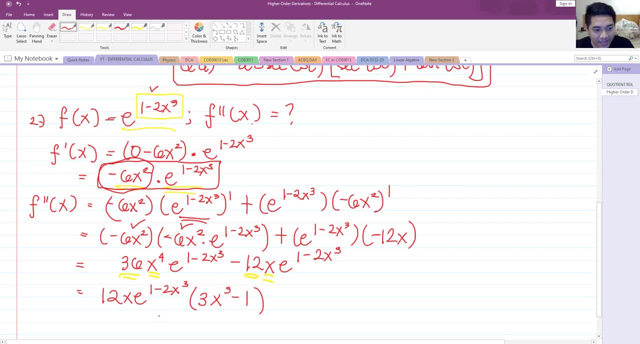 1. so if we factor this out, if we distribute 12x e raised to 1 minus 2x cube to 3x cube, the, the result will be 36x raised to 4 e raised to 1 minus 2x cube. okay, so this will be our final. 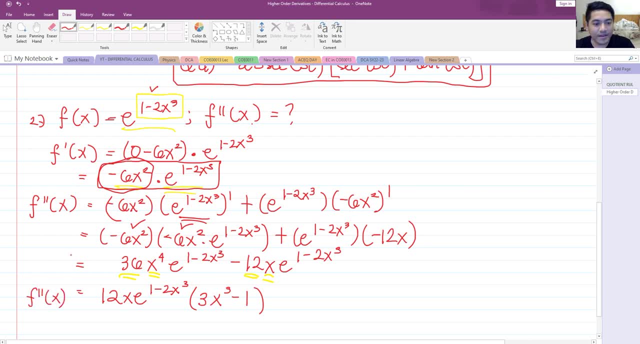 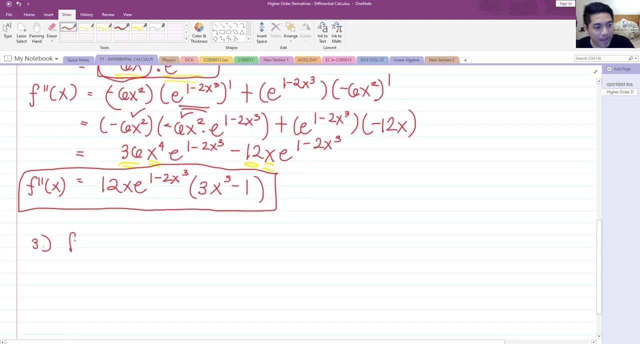 answer for the second derivative of this function. okay, so that's the second derivative. okay, so how about for another problem, number three? okay, so for problem number three, we have f of x equals ln of 1 plus x squared. okay, and then we're going to get the f double prime of x. 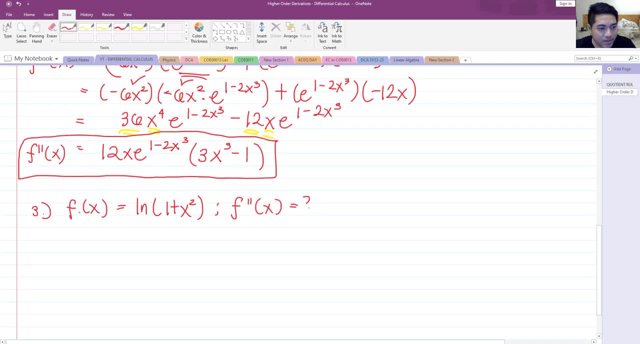 okay. so let's try to solve this. so first, derivative: okay. so in getting the ln, let me just recall, we differentiate first whatever is inside the ln and divide it over the original function inside the natural logarithm. so again to recall, we have d all over dx of ln of x. first we need to differentiate x, okay, divided by the original. 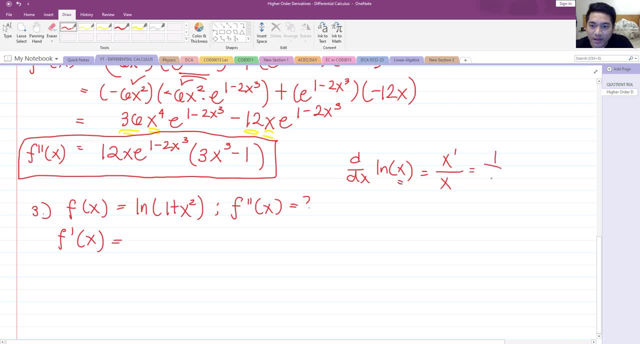 function which is x. so the derivative of x is 1, and but divided by the original function, we have 1 all over x as our answer. so in this situation it's still the same. so first we have to differentiate 1 plus x squared all over the the same function, which is 1 plus x squared. so 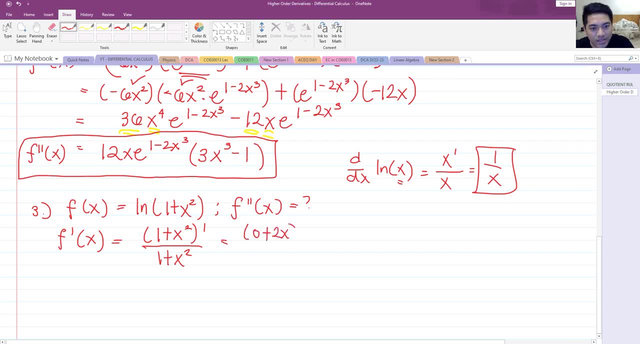 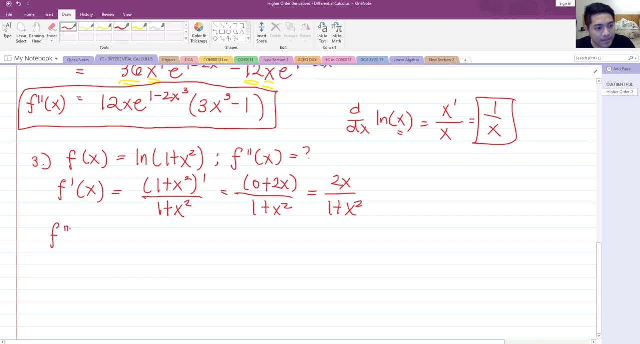 differentiate 1 plus x squared, that's 0 plus 2x all over 1 plus x squared. or that's simply 1: 2x all over 1 plus x squared. so that will be your first derivative. okay. so how about the second derivative, if we are to repeat differentiation? okay, with the first derivative that we have gotten. 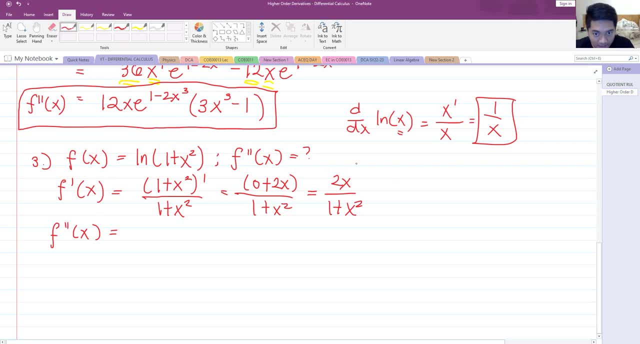 okay, we will be having a quotient rule, okay, so the quotient rule. so the quotient rule is low d high, okay, minus high d low, all over low squared. so i have taught that formula okay on my previous discussion about the quotient rule and here it is just a quick. 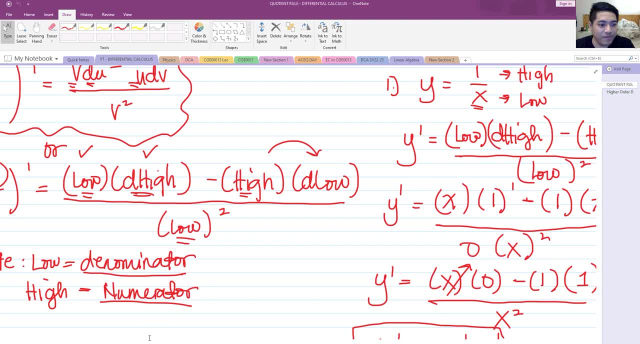 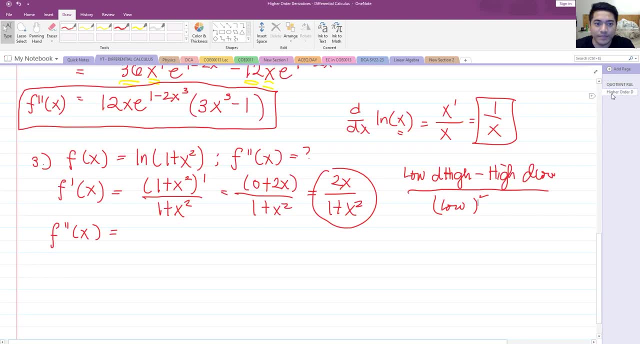 snap, okay, this is the formula for the quotient rule. so we have low d high, minus high d low, all over low squared, so we're going to use that. so low we get low 1 plus x squared. that's the denominator and the differentiate, whatever is the numerator. we have 2x and then minus, okay, minus high, which is. 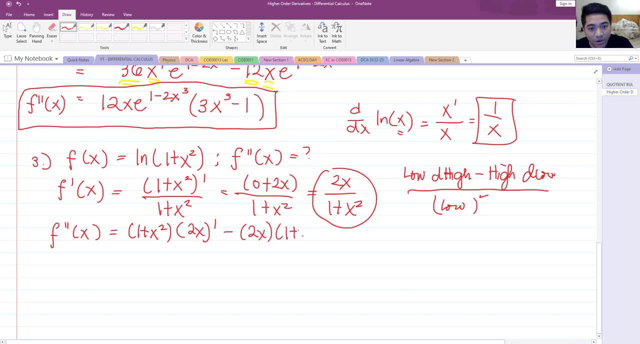 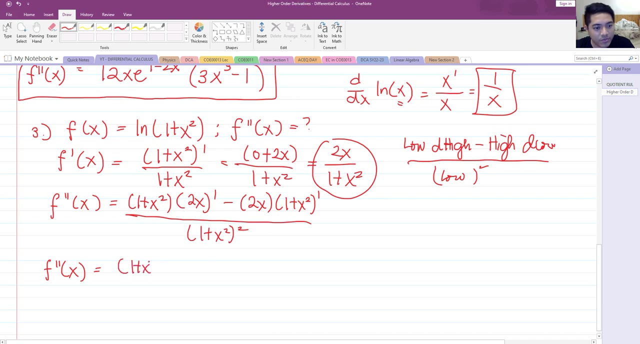 the 2x or the numerator and differentiate the low. okay, and all over we have to square. whatever is the denominator, all right. so we have f double prime of x, so that we have 1 plus x squared. multiplied by 2x, that's 2 minus 2x. then we have 1 plus x squared.